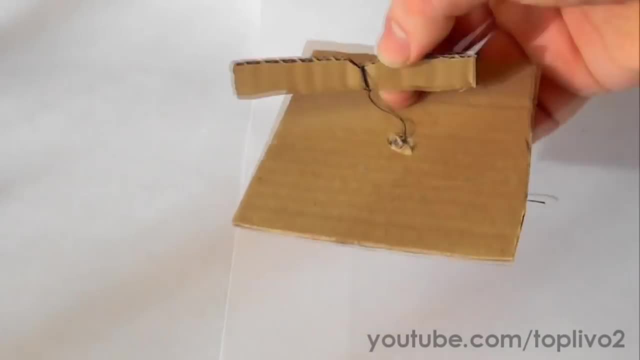 To do this. I came up with an interesting system in which you can conveniently choose the right thread. To do this. I came up with an interesting system in which you can conveniently choose the right thread, conveniently change the height of a crystal. Also, with this system, the cup is. 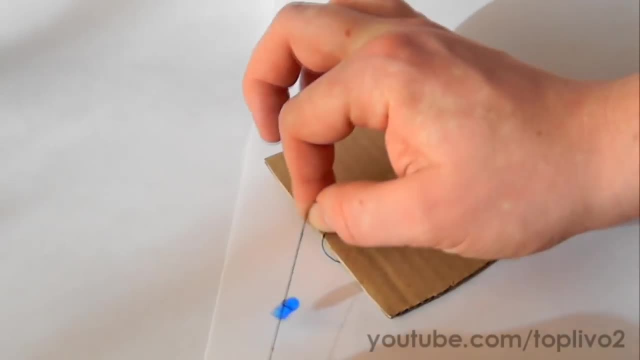 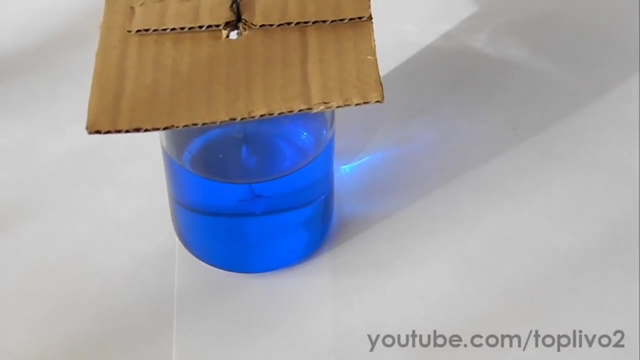 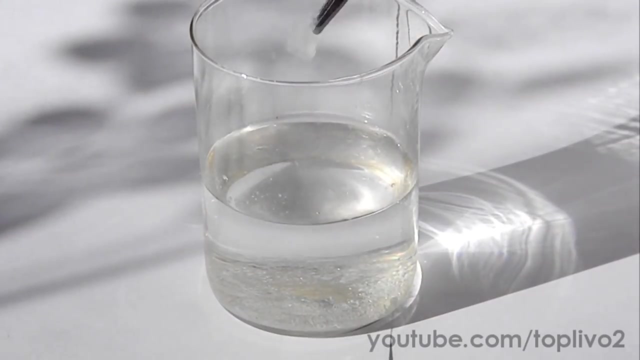 protected from dust. We hang the crystal to a cup and now all we do is wait. Growing crystal requires a lot of time and patience. When I was doing it before, I was also growing a crystal of a mixture of potassium chloride and sodium chloride in parallel with making the crystal of copper sulfate- Here the 60%. 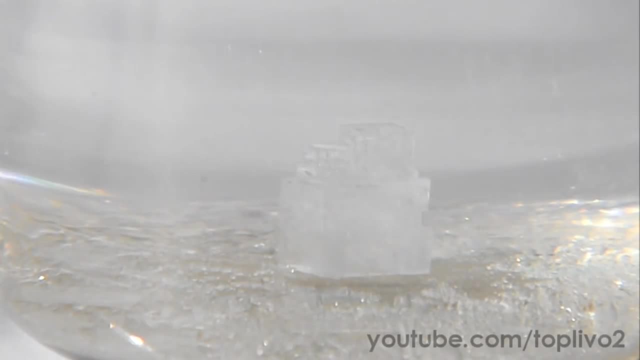 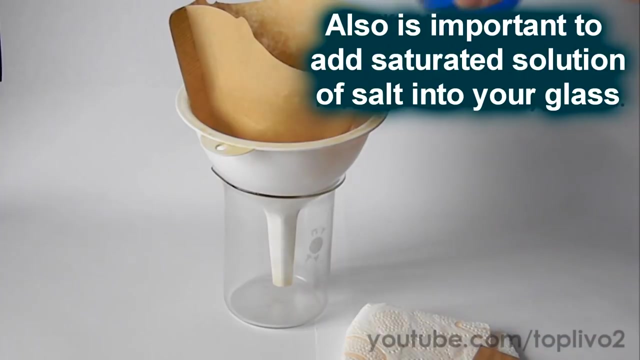 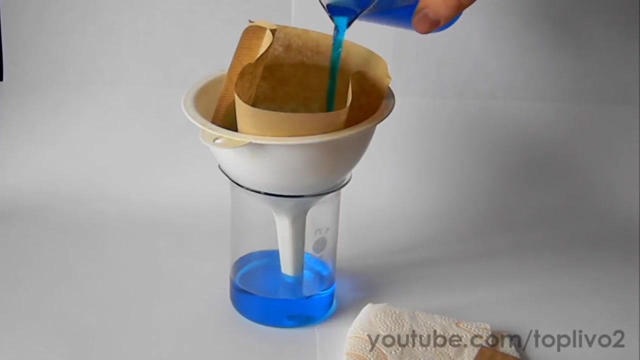 of potassium chloride and the rest of just sodium chloride. If you want to get a very smooth and beautiful single crystal, you'll need to fill the solution every two weeks to maintain its cleanness. If the solution is dirty, a crude crystal will grow and you'll get a polycrystal instead of a single crystal. 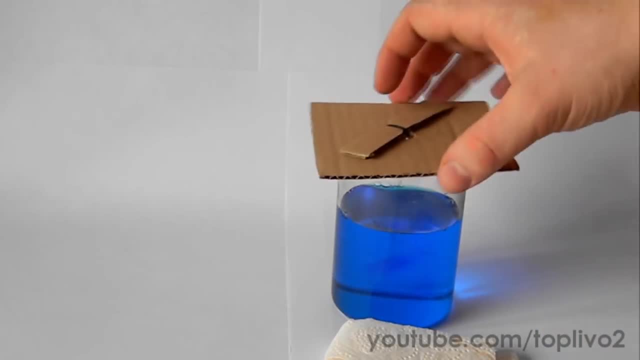 we want. Polycrystal is when a lot of crystals fuse together. Now I'm going to show my crystal grown stages. Sorry, I've not filmed up to the end of this video. If you liked this video, please subscribe to my channel. 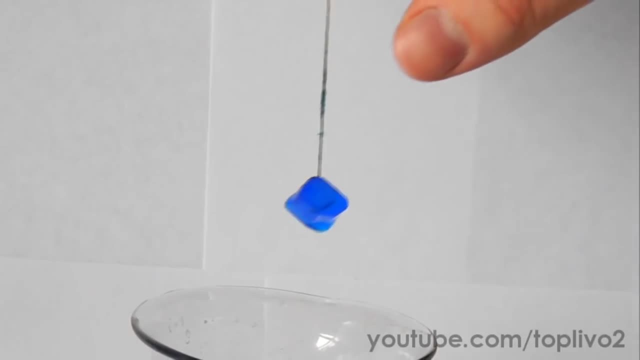 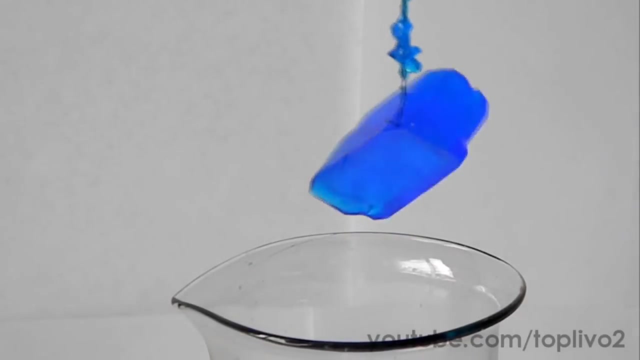 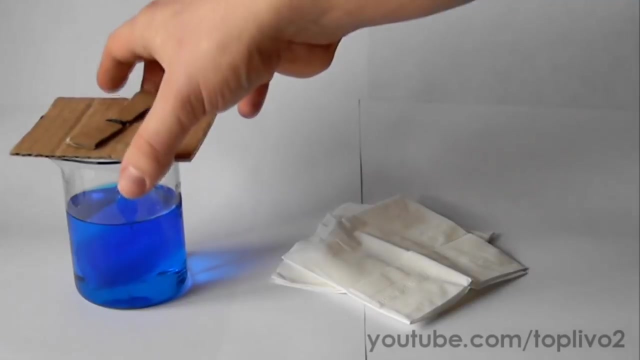 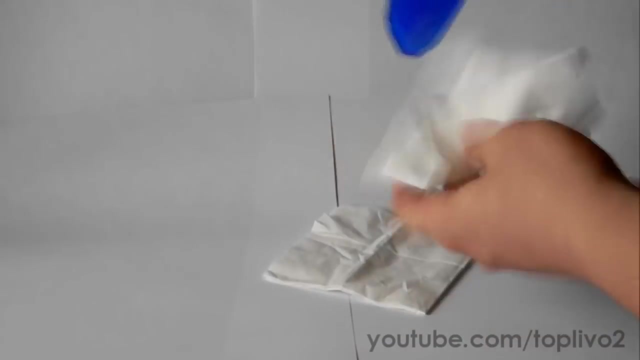 The first week, second week, third week, fourth week and so on. After two months and one week, I've decided my crystal was big enough, so I want to stop its growth And to do that, take off the crystal from the solution and dry the surface using a cloth. Next, you will need to cover the 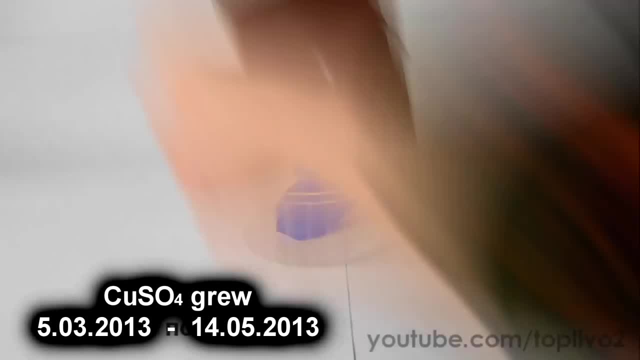 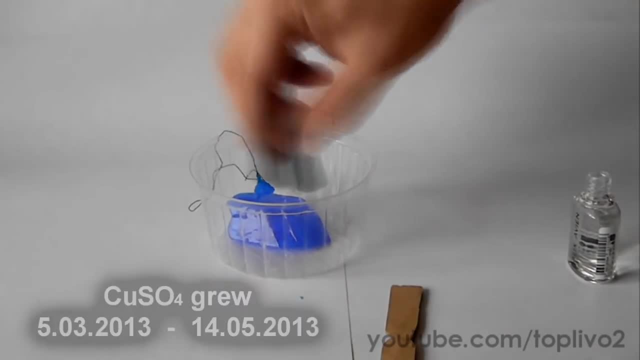 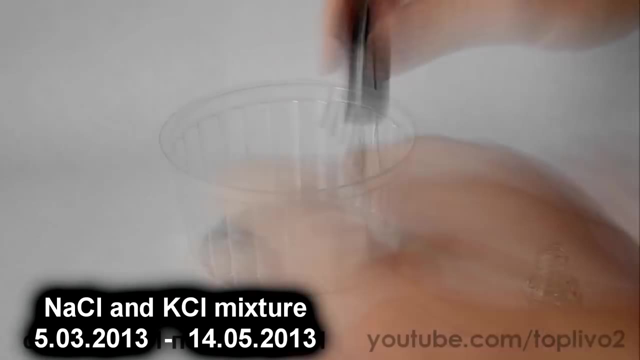 crystal with colorless nail polish. One or two layers is enough. It is necessary to protect the crystal from further destruction. My second crystal mixture of sodium chloride and potassium chloride has grown a node. I'm covering its surface with lacquer. After the lacquer has dried, the crystal can be tanked with bare hands. As you can see, the crystals are very big. 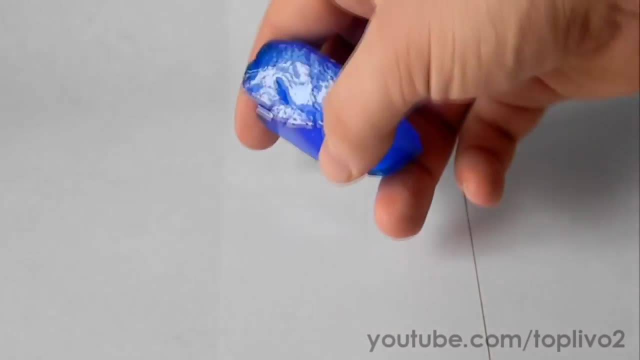 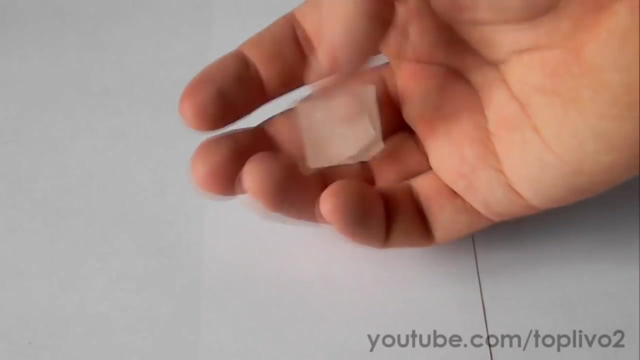 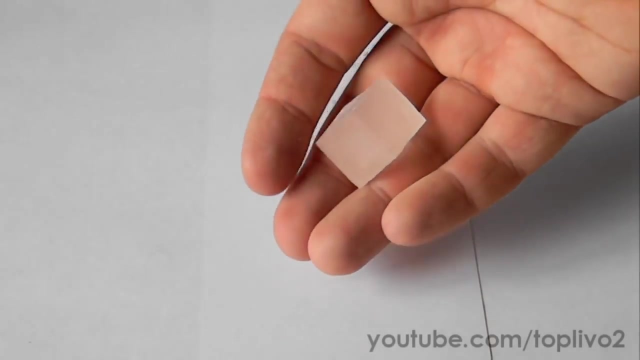 As you can see, the crystals are very big. As you can see, the crystals are very big, Beautiful and quite smooth. And now, ladies and gentlemen, as we have done a long journey growing these crystals, Let's just enjoy their beautifulness without any further comments.